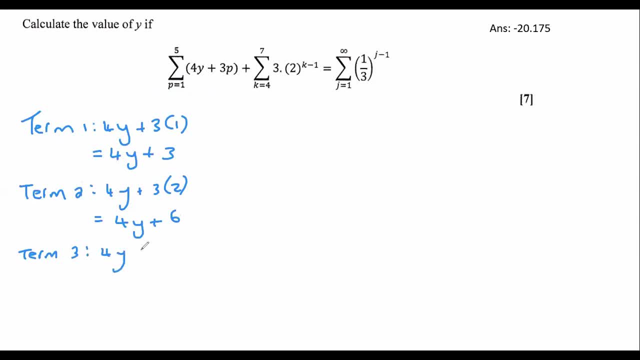 by plugging in a three, And so that's going to be four y plus nine. All right guys. so what we now do is we can have a careful look at term number one, term number two and term number three. Okay, and you need to try and identify. what are they doing? Are they adding? 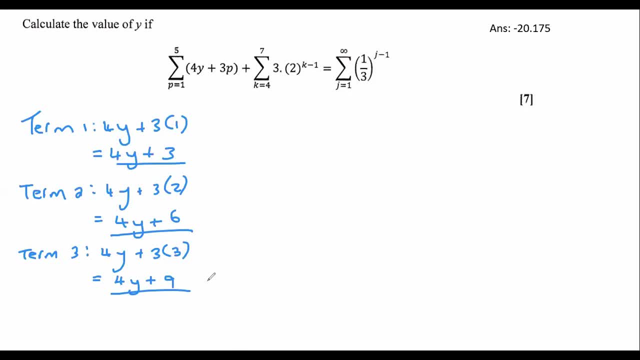 Are they minus? Are they missing? Are they multiplying? What is going on? Well, most of you should be okay with the fact that it looks like they're adding the number three. You see, if you go from four y plus three, then if you add three, that'll give you four y plus six, And if you take four y plus six, 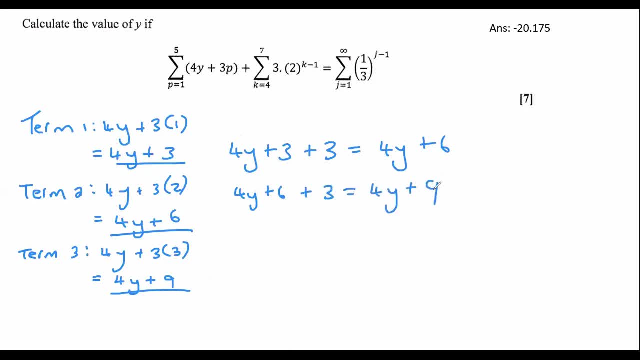 and you add three, you're just going to end up with four y plus nine. So what we can then say is that that part over there is arithmetic. Okay. so let's quickly do that. Let's put a box around this one. 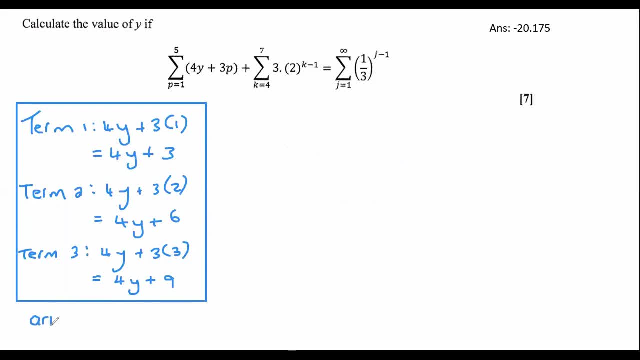 And then we can say that this part over here is arithmetic. And what's the common difference? The common difference is three. Excellent, Now what I'm going to say now. I'm going to stay with this one over here Now. 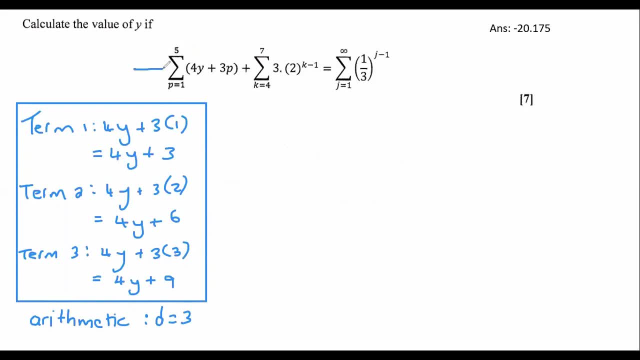 did? you guys obviously know that this thing, the sigma notation. what does it actually mean? It means the sum. of It means the sum of Now. there are only going to be five terms in the sequence. How do I know that? Because we are counting from one up to five. So 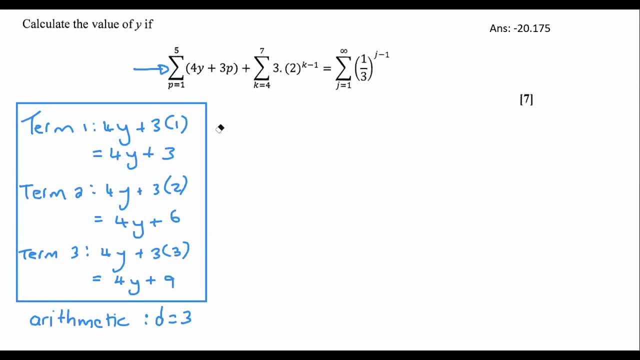 that is five terms. So we might as well go and calculate term four and term five quickly. right, You can put it into the sum formula. But if there's only five terms, I think we can just do it manually. We don't have to go get the formula and all of that stuff. 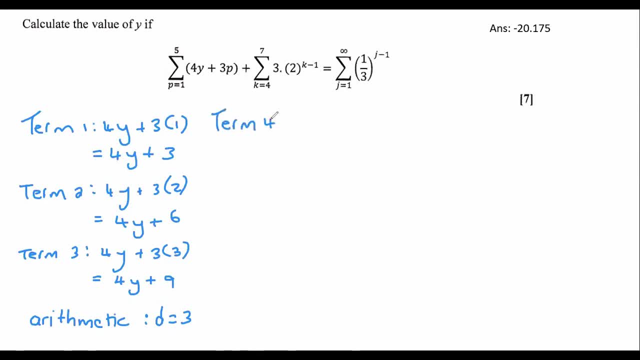 So we can just go get term four quickly. So I'm still busy with this one. So term four would just be like that, And that would give us four y plus 12. And then term five would just be four y plus three times five, And that would be four y plus 15.. Excellent, So we. 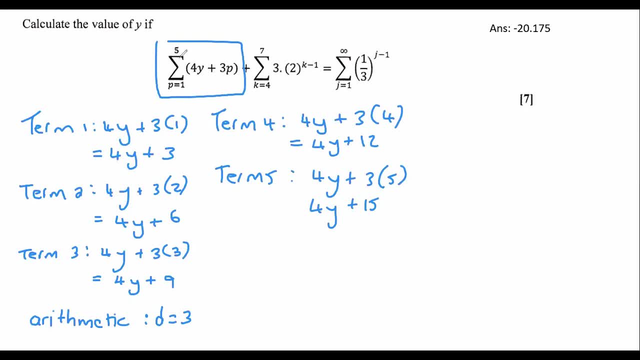 have all five terms. And what does sigma notation stand for? It means the sum of. So we can just go add all of those together. now We just add term one, term two, term three, term four and term five, And so 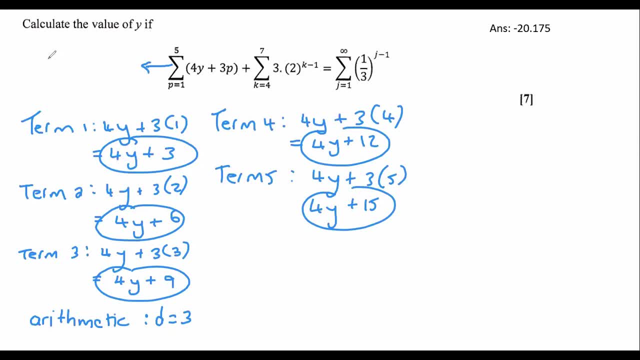 if we're to go and do that, we should end up with 20 y plus 45. Let me just double check that. Yeah, You should end up with 20 y plus 45. And then, if you wanted to do it with the formula, 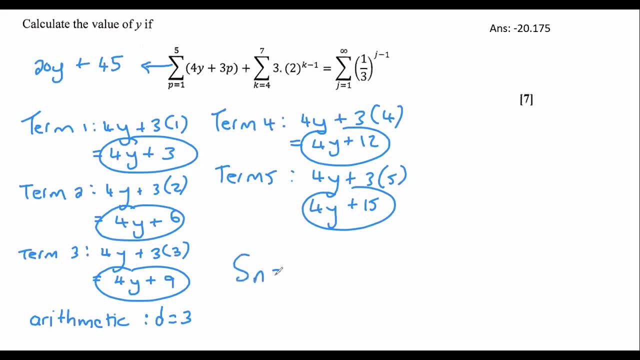 then you could use the formula Because it's arithmetic. you would have used: s n equals to n over two, two a plus n minus one times d, And you could have used that formula for this over here as well. You will eventually get to 20 y plus 45.. The only reason I did it: the manual. 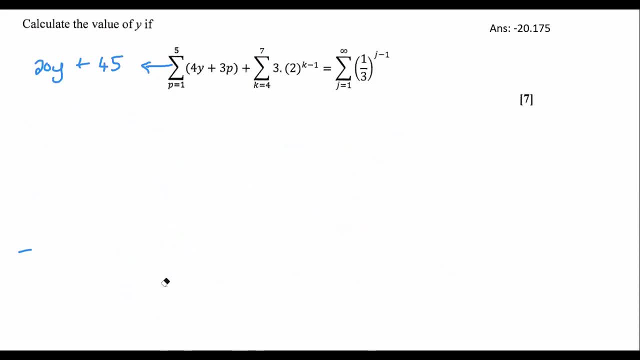 way is because there were only five terms. But if there were like 45 terms, then obviously we would have used the formula. What I'm now going to do is I'm moving on to this part over here, Okay, And once again I'm going to go do the first three terms. Why? So that I can see what type of 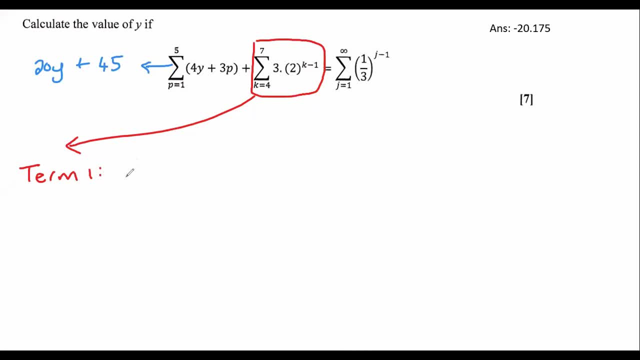 sequence we are busy with. So how do I find term one? I take this number that I see at the bottom and I plug it into the equation. That number doesn't have to be a one, guys. That's not what it means. 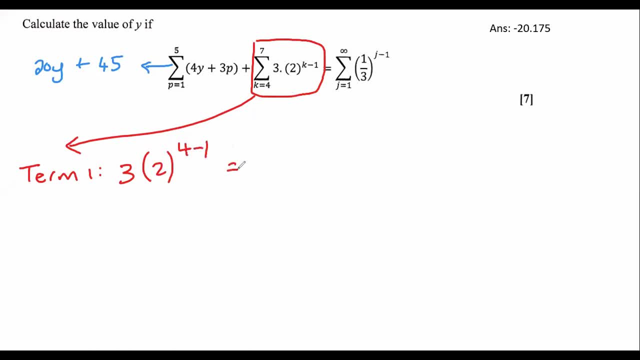 So I'm just going to plug it in on my calculator as I see it like that, And that gives us 24.. I don't actually think this is going to be a very difficult question. I think it's just long. to be honest, It's not difficult. We're literally just plugging in formulas here. 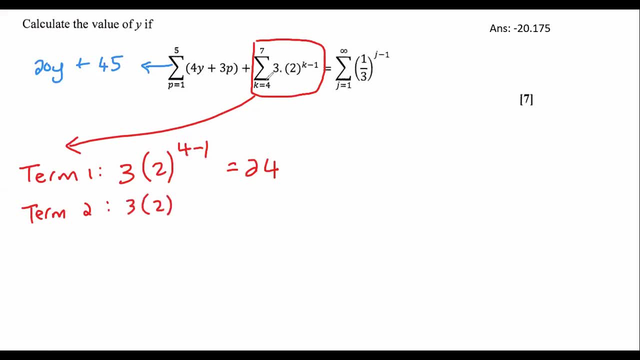 Term two: we're just going to increase this number by one, So that would take us to a five. All right, 48.. Then I carry on term three. How do I do that? I just increase that number another one, So that's going to be a six this time. 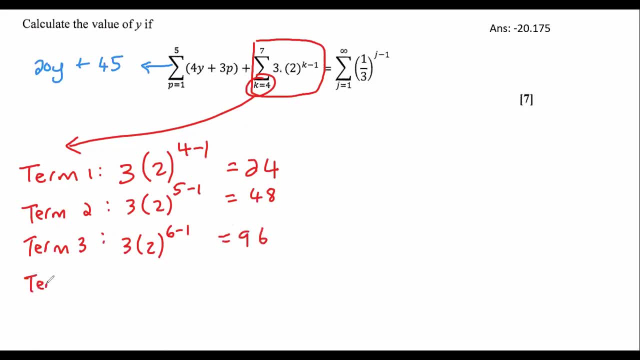 and that's going to give us 96.. And then I might as well just go one more, because that will take us up to the seven over there. That'll take us up to the seven. You see, we counted from the four up to the seven. That's all that sigma notation actually is. 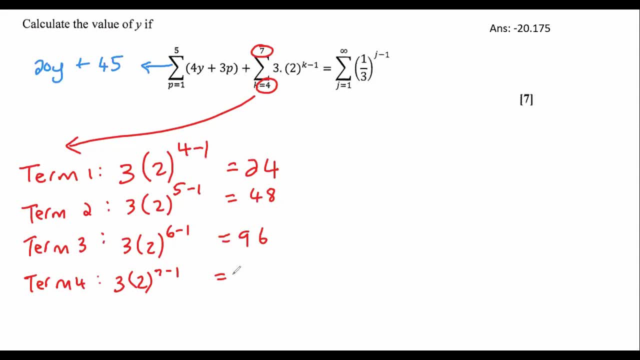 And that should give us, I think, 192.. Yes, 192. 192.. And then I'm just going to add all of these numbers together, these numbers over here, Just going to add them, And that's 360.. All right, And now I'm just going to go do the last little part. 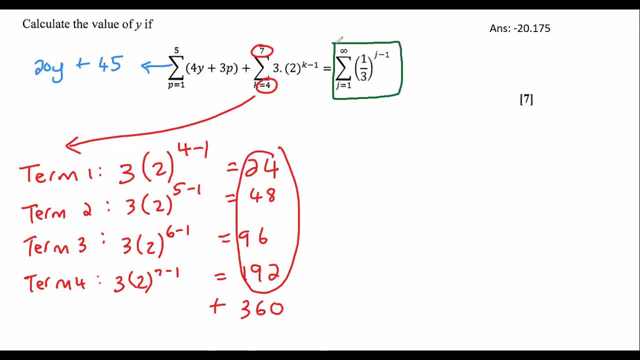 which is this part over here. So I'm just going to go find the first three terms. I know it's going to be geometric. Why do I know it's going to be geometric? Because they have a little infinity zone. They don't have any number, but they are going to have a little infinity zone. 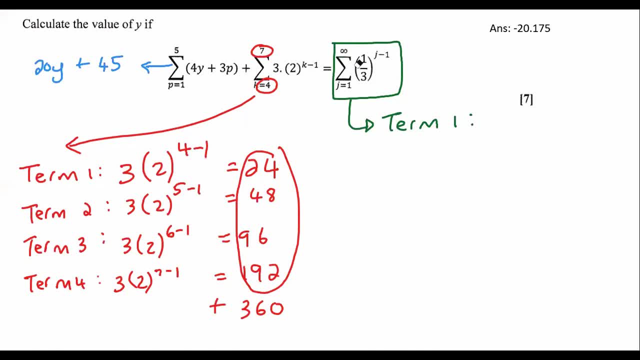 symbol at the top and you can only use the sum to infinity on a geometric sequence. Exactly, Kanye. Kanye made a good point. They catch you by making it look difficult. So, guys, my rule for you guys- or not my rule, but my advice is when you see something like this: 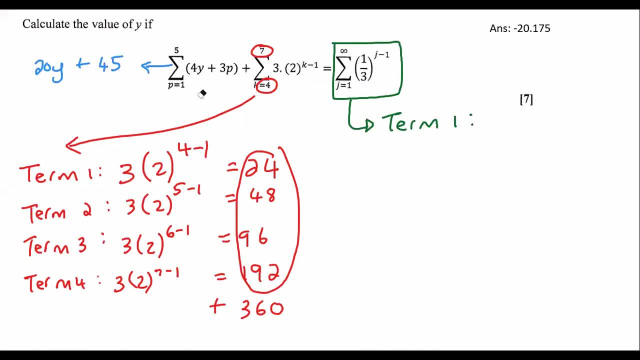 it looks terrible, I know, But, guys, I promise you, I've seen so many of these types of things and what I've learned over the years is: just start with the question, plug in the information, do what you can, and it slowly starts to unfold itself. There are some questions that you will. 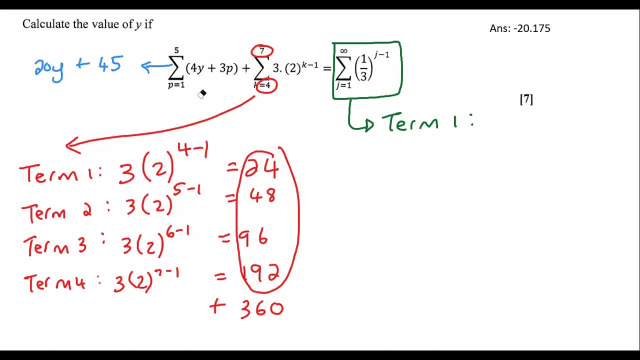 get stuck and you'll look at it and you'll be like, okay, now I don't know where to go. But most of the time you should be able to just start the question, and then you might get stuck somewhere in the middle, but at least then you'll get some of the marks, Okay. so just start the. 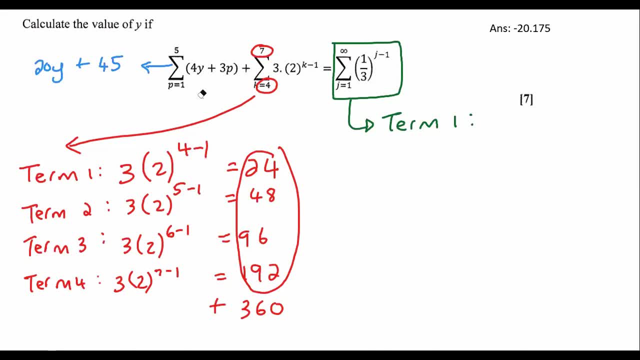 question. let it unfold and move on. Most of the time it's just going to get to an answer. That's the beauty of maths: It just gets there somehow if you just follow the basic rules. So yeah, it's very difficult to go very 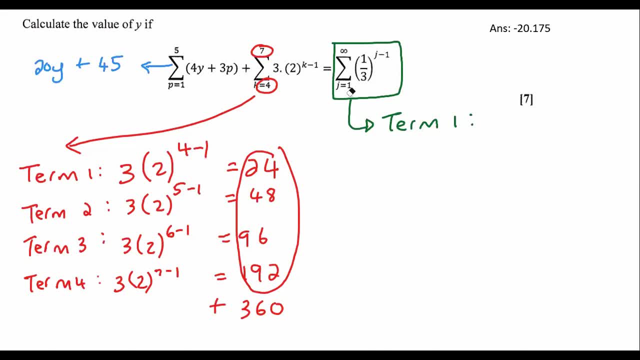 far off track. if you just start the question and you do what? yeah, okay. So if we find term one, term one, we're just going to plug in whatever number is here at the bottom, And so that is a one. That's just a coincidence. It doesn't have to. 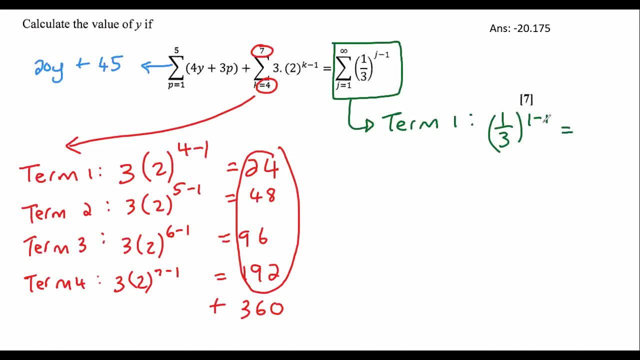 And so I'm just plugging in a one and that's going to give us a one. Then I'm going to plug in term two. So you must never be put off by what the question looks like. I've seen some really difficult looking questions like this is one of them, and it's actually such a joke Like this is. 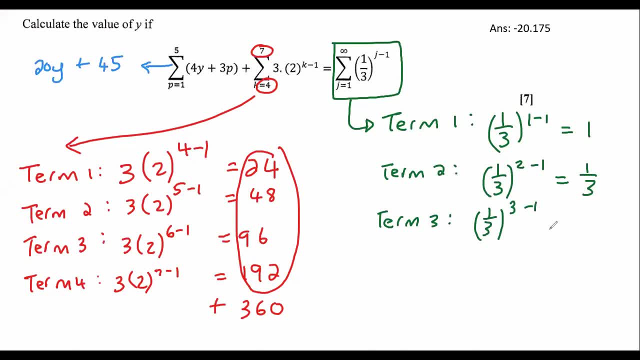 just a big joke right now, Like we're just filling in stuff And if we do that, that should give us one over nine. Okay, We can't go add all of these together, because we would never stop, because it's a sum to infinity. 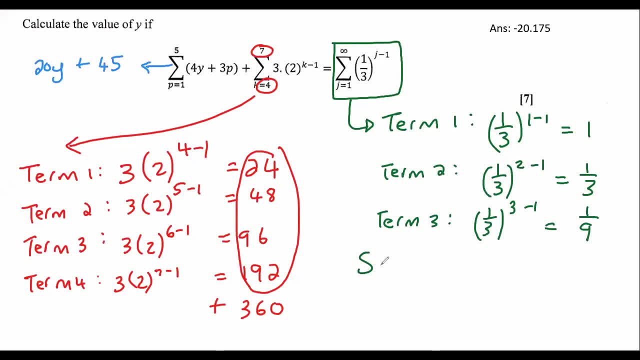 So what we're now going to do is we're just going to use the sum to infinity formula. Remember that one A over one minus R. All right, Uzair, let's see what happens. Let's see what happens there. So this answer I just got. 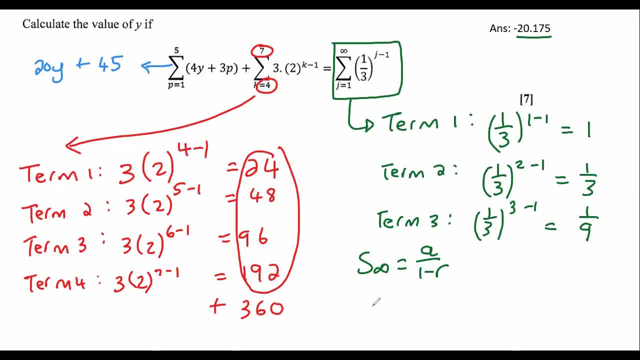 from the memo. but hey, memos can be wrong as well. So let's see what happens. So we need to get a value of R. Now, to get an R value, you're just going to take term two, term two, and divide it by term one. 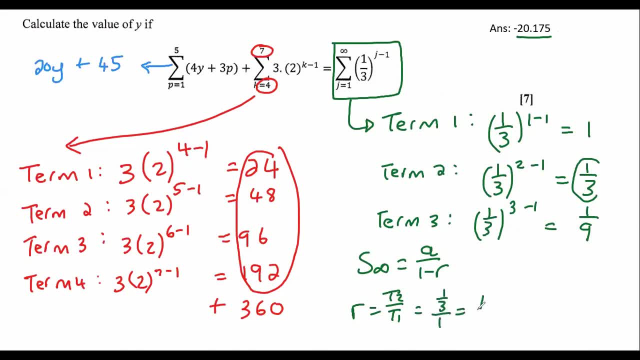 for example, and that's going to give you a third divided by one, which is just a third. Okay, guys, I'm just switching off my video for a little bit, Probably getting in the way right now, So I'm just going to put that off, And so now we can go get the sum to infinity. 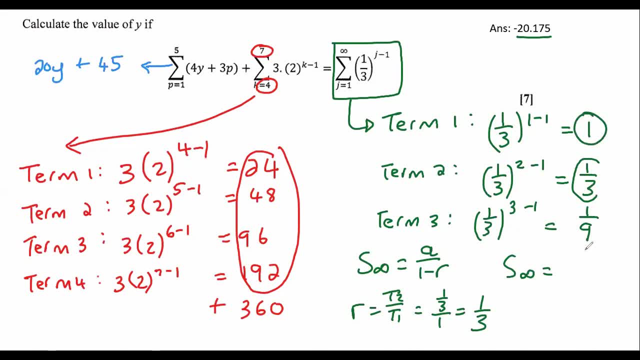 and that's going to be A over one minus R. So A is term one, one minus a third. And this should be what's that? Three over two, One over one minus a third, Three over two. Well, I'm just going to say: 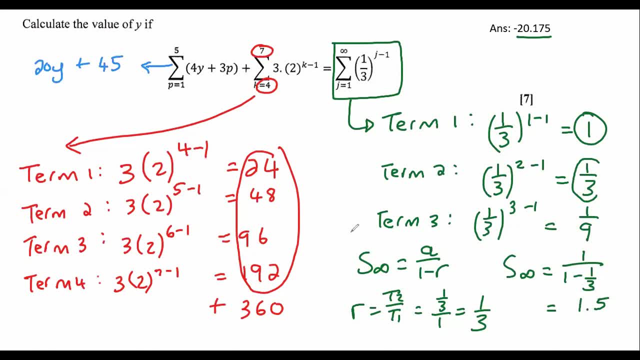 1.5.. 1.5. And so now we're literally just going to go plug everything in. So the first part here is 20Y plus 45. So we're going to go 20Y plus 45. Then the red part. this part here was 360.. 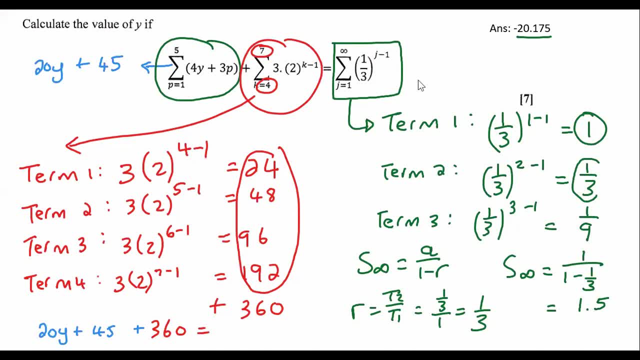 And then that's equal to The part that was in green, and that was 1.5.. And there we go, guys. Now it's just a matter of solving. Let's clear up a bit of space here for ourselves, And so I'm just going to solve.